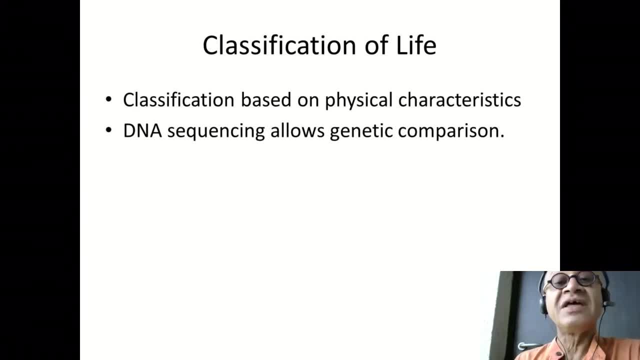 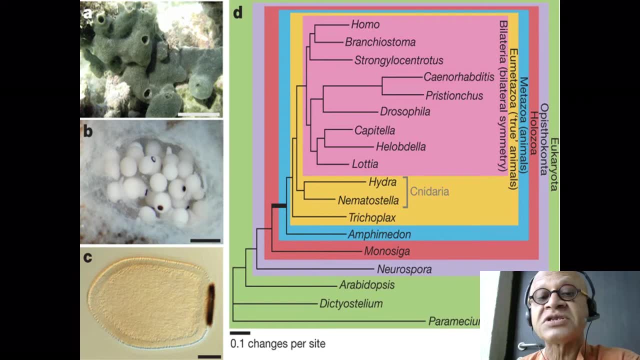 So DNA sequencing now has obviously gotten into genetic comparisons and classifications. So just a brief introduction here. If we want to look at the origin of, let's say, our species Homo sapiens, we know we had some ancestors like Homo erectus. 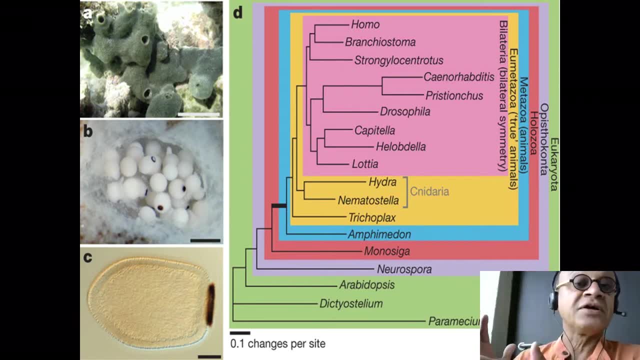 Homo habilis and we split off from. we had Neanderthals as our relatives, but we split off from earlier so-called hominids which were also walking on two legs, like Canianthropus, Australopithecus, Ardipithecus, and so on and so forth. 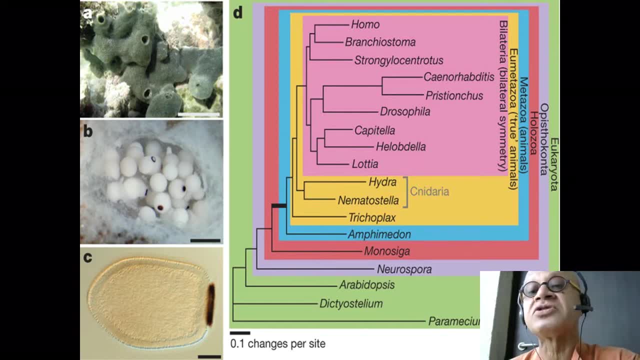 But this is going much further back. so it's going to show us if you keep following the genetic markers in what is called a molecular record, if you keep following the genetic markers in what is called a molecular record, in what is called a molecular record, if you keep following the genetic markers in what is called a molecular record. 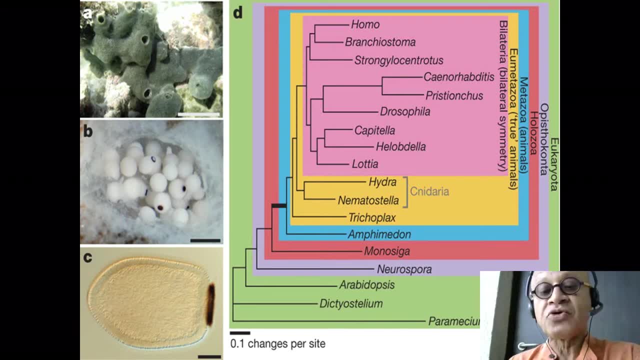 if you keep following the genetic markers in what is called a molecular record, then where do we all originate from? So you can see, there is something called paramecium, which is like a sponge- marine sponge- which can be traced as the origin. 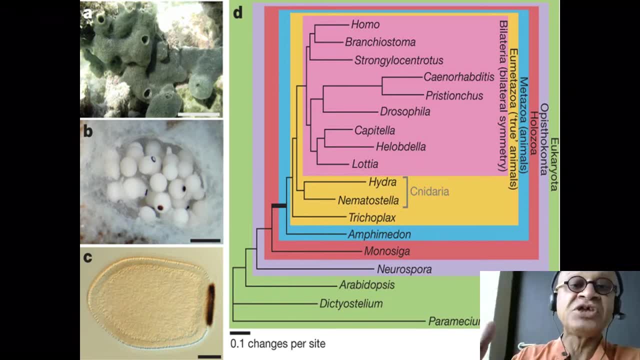 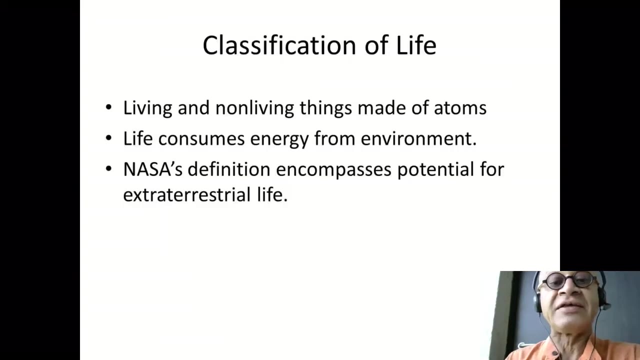 So the evolution happens with mutations and adaptations and response to the environment and so on, And newer species have evolved over time. but we are all kind of related. so we are all kind of related. but we are all kind of related and we can't really go back genetically. 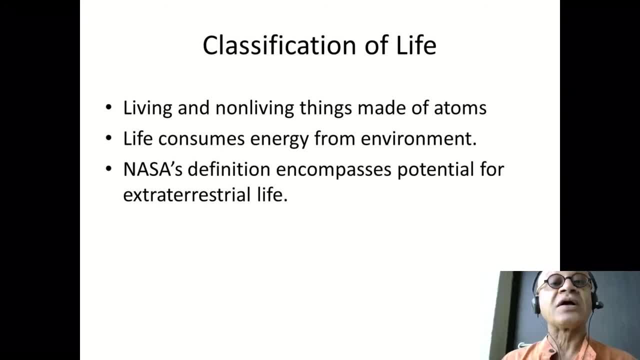 So living and non-living things are made of atoms. So if you think about our body being made of carbon and water and you have CO2 going in and out of the body right as we breathe out and produce CO2 in the body, 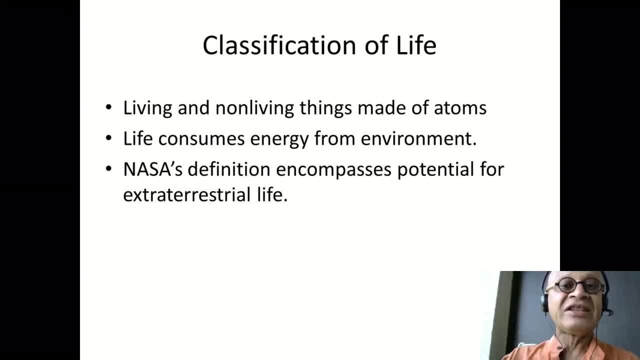 water is going in and out and so on. So atoms are kind of the continuum from inorganic to organic matter. So atoms are kind of the continuum from inorganic to organic matter. thing that we will see is defining life is not that straightforward, but life 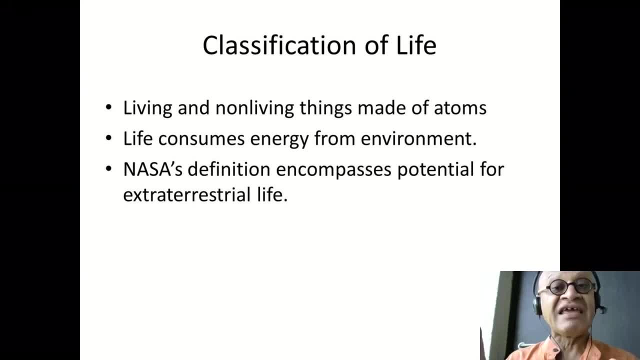 consumes energy from the environment, which means life produces waste. is that enough to define life? not quite, okay. NASA's definition encompasses the potential for extraterrestrials life, life. so NASA is interested in what is called astrobiology. so they want to see if there is life on other planets, right? 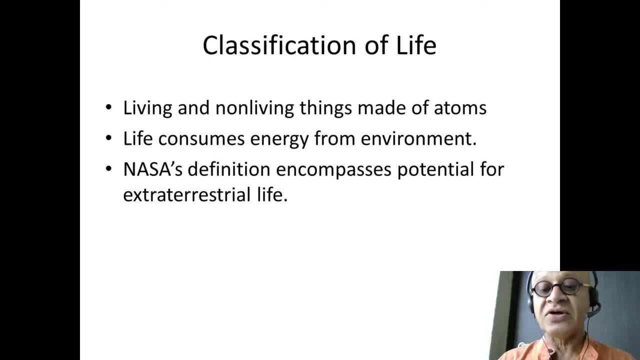 obviously you might have read just recently, as I'm recording this- just last week. there is some evidence that the atmospheric component called phosphine has been detected on Venus and on Earth. as far as we know, phosphine can only come from biotic activities, so the exciting news is that maybe Venus has some sort of microbial life. 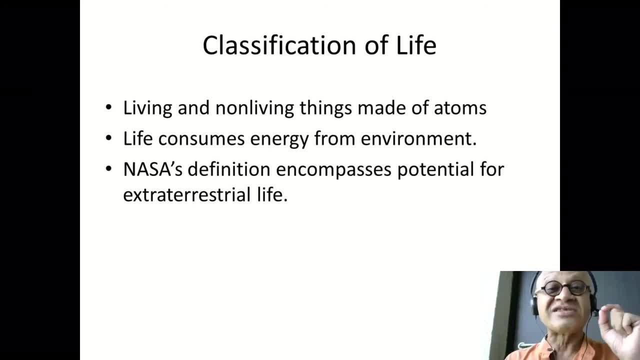 remember, Venus has surface temperature of four hundred and sixty degrees. that's hot. so on earth, in fact, you go and look for extreme environments where things may be living, and one of the extreme environments actually occurs in the ocean, called the hydrothermal vents. will look a little bit at it. sulfuric acid. 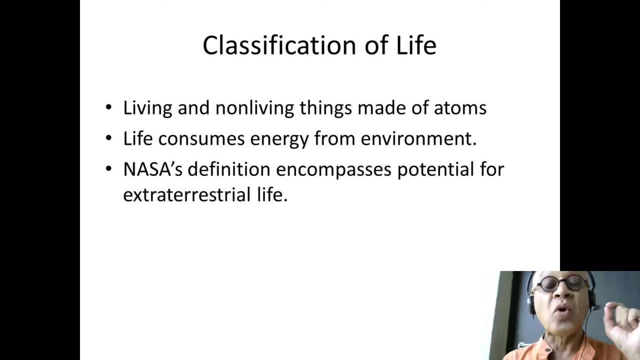 very noxious, toxic, warm hot water gets produced, but yet hydrothermal vents are full of life forms. so life again finds loopholes to survive in extreme environments. so NASA looks for life in extreme environments on earth so that it can go outside and detect life on other planets. so the definition of life for NASA has to. 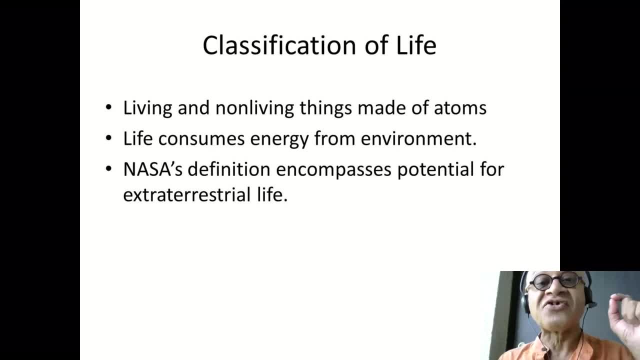 include potential for extraterrestrial life. ok, so we going from marine life to life, definition of life, extraterrestrial life and so on, but all related. 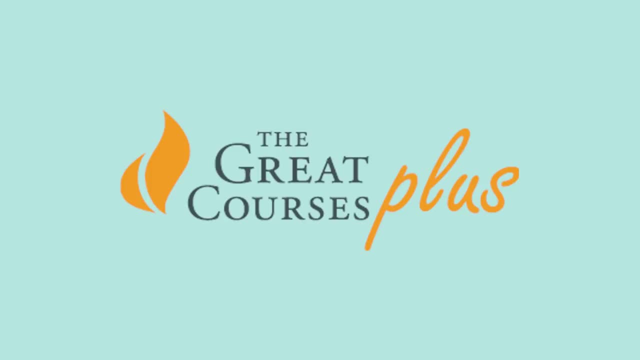 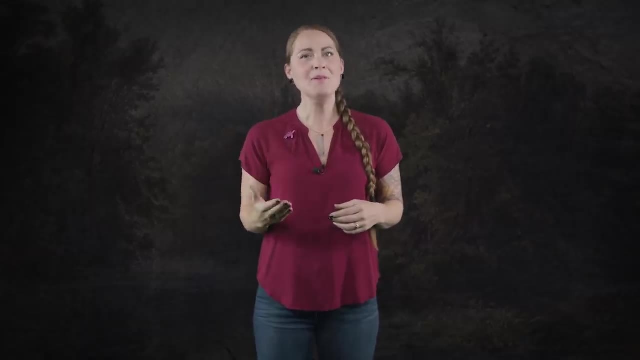 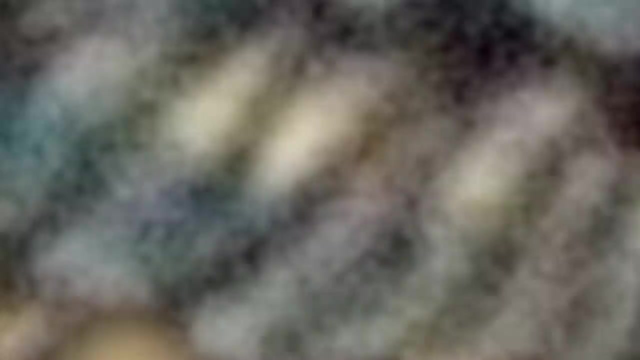 This episode is supported by The Great Courses Plus. Even though we often refer to this time in history as the Age of Mammals, we should probably be calling it the Age of Insects, Because just looking at the numbers, there are way more of them than there are of us. 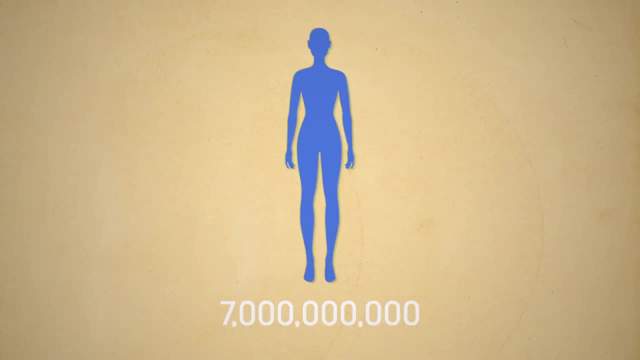 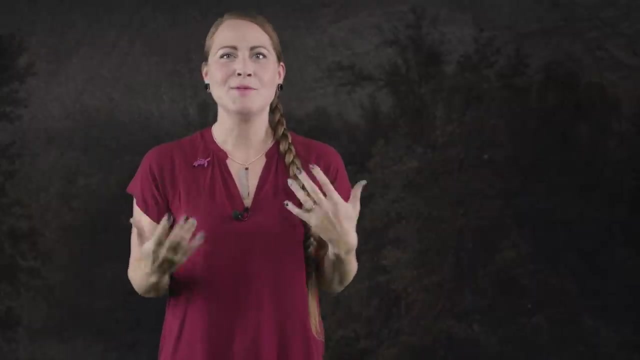 Humans alone number more than 7 billion at this point, which is a lot, But insects Try 10 quintillion. We may like to think we're in charge because we make the rules, and well, we're bigger than they are.